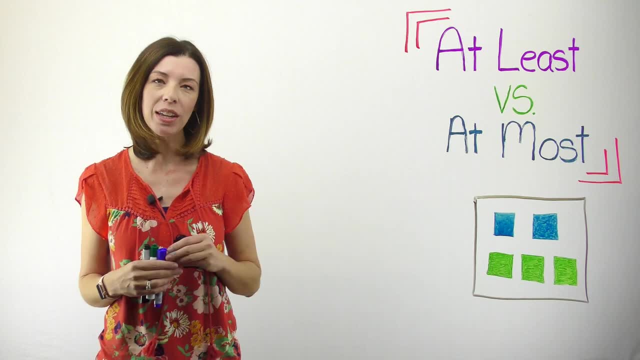 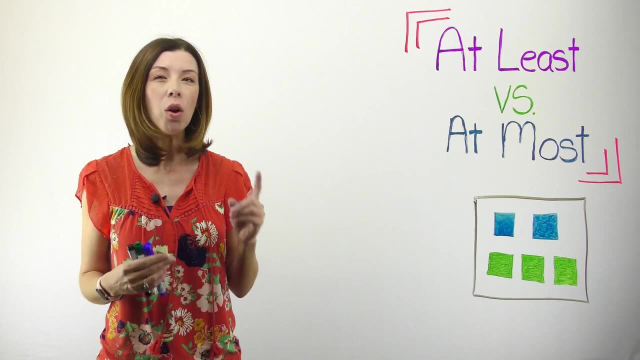 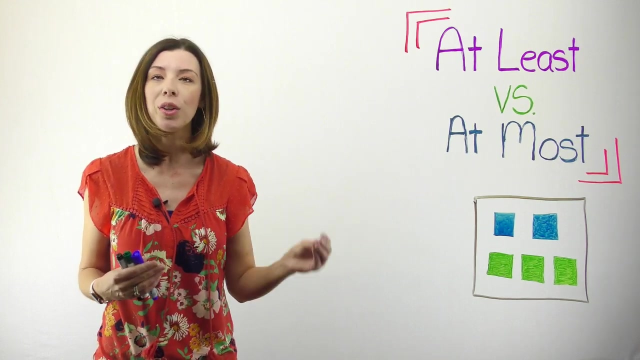 now we're talking. If I say you can have at most one cookie, then are you allowed to have two cookies? No, At most you can have one cookie. Your only option is to really have one. But are you allowed to have NO cookies? if I say you are allowed to have at most one cookie? 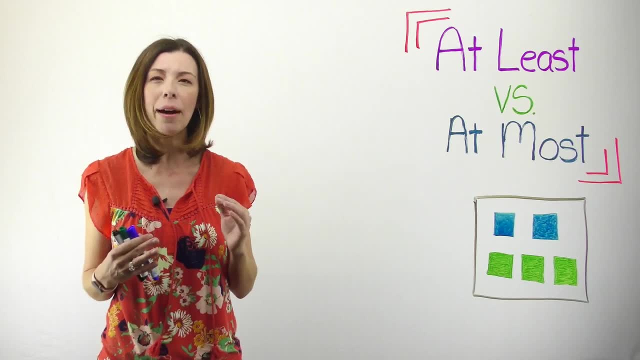 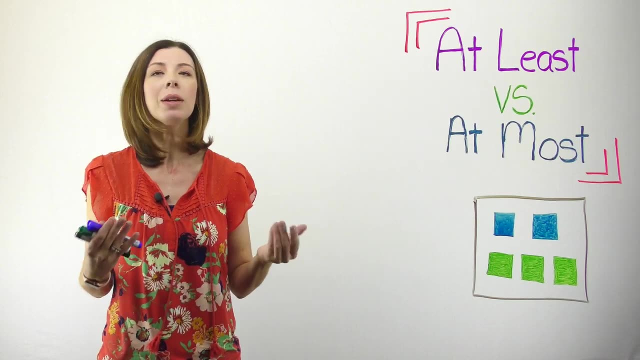 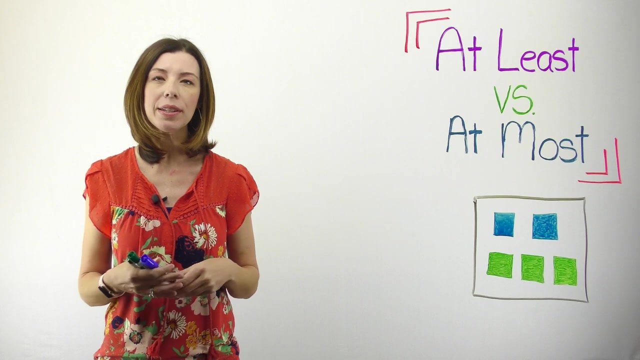 Yes, You could have zero cookies. You have to think about these problems in terms of what are the possibilities in which you could win. If somebody was saying, what's the probability of pulling out at least two blue cubes, Let's think about what are all the possibilities that we could win. 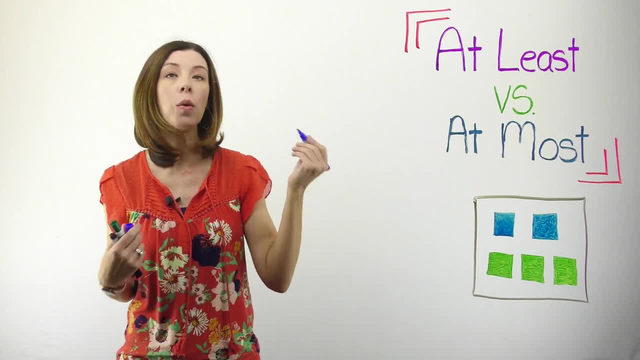 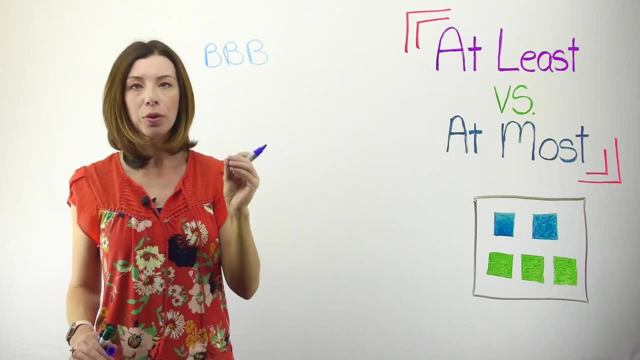 So if we say at least two blue cubes, I know that one possibility is I could have a blue, blue, blue right, At least two blue cubes. So I'm still winning if I get three. Okay, let's think about another possibility. 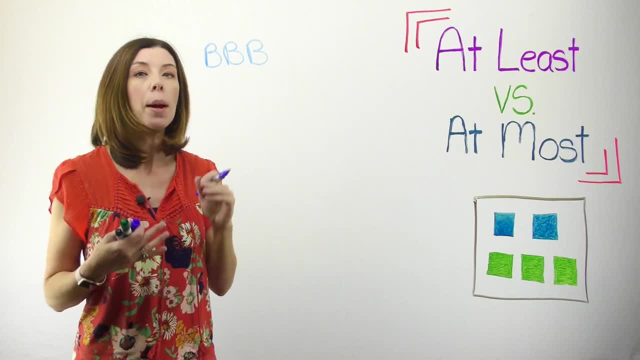 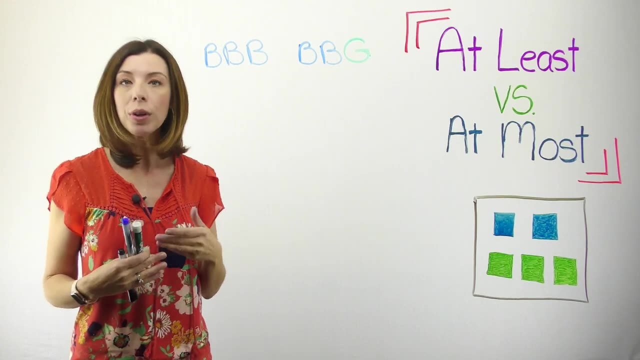 I could also just get two blue cubes right, So I could get blue, blue and then green. If I'm thinking about pulling these out one after the other, I could also think about green, blue, blue, right, If I get a green first and then two blues. 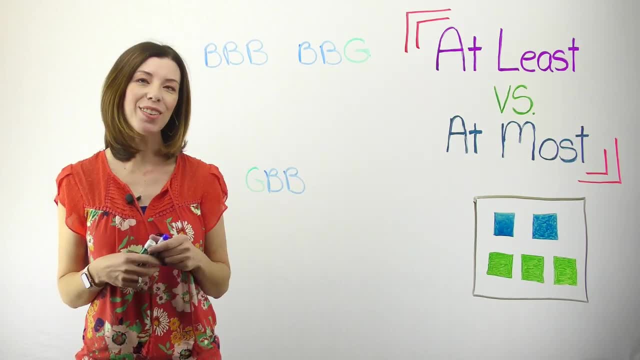 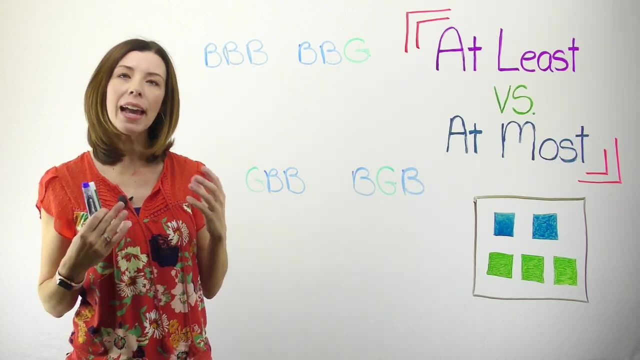 that would also work. The last scenario that I could get would be if I got a blue, then a green, then a blue. The next step I have to do for this problem is I have to figure out the probabilities for each scenario. I'm trying to find that probability. 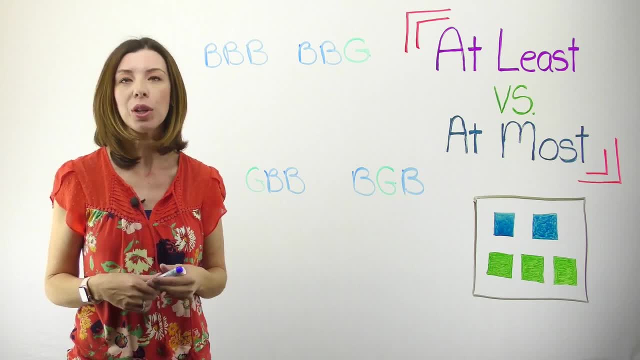 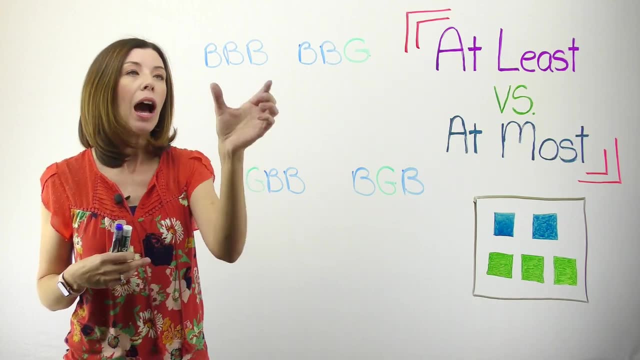 of pulling at least two blue cubes, Because these are independent events. right, I'm putting the cube back in before I pull the next cube. I'm going to be multiplying with the probability of pulling two blue cubes, So I'm going to be drawing three different probabilities here. 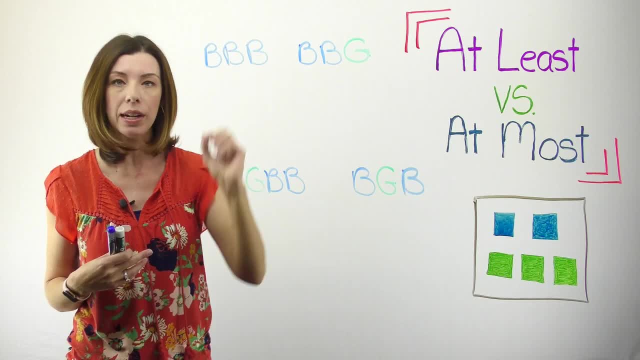 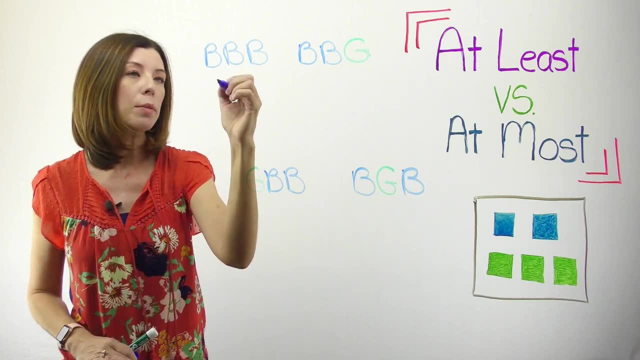 in order to find the whole probability for this one scenario. So you can see I've got my cubes here and I've got two blue cubes out of five, So I'm going to go ahead and write that my probability for drawing the first blue cube. 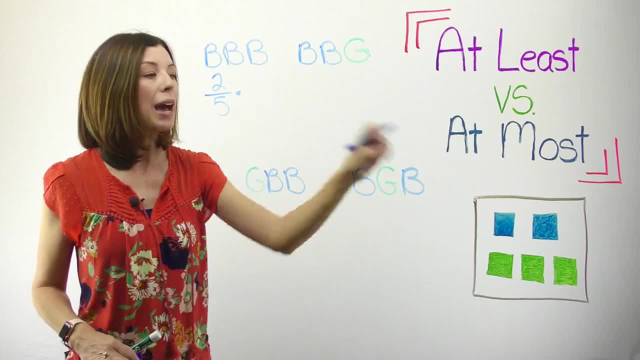 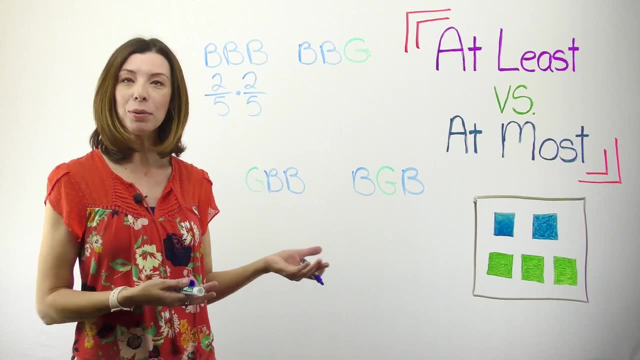 is two-fifths. Now again, I put it back in: My probability for the next blue cube is going to be also two-fifths. My probability for my third blue cube is also two-fifths. Next I'm going to go to my next blue cube. 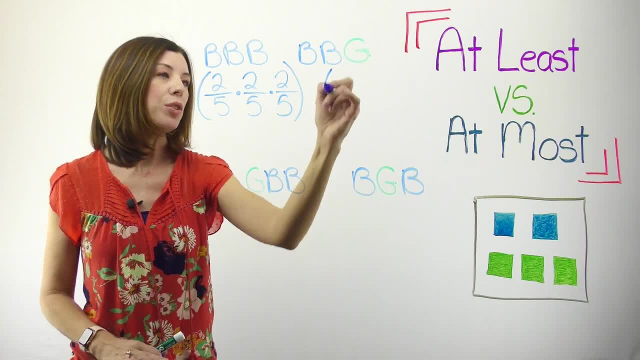 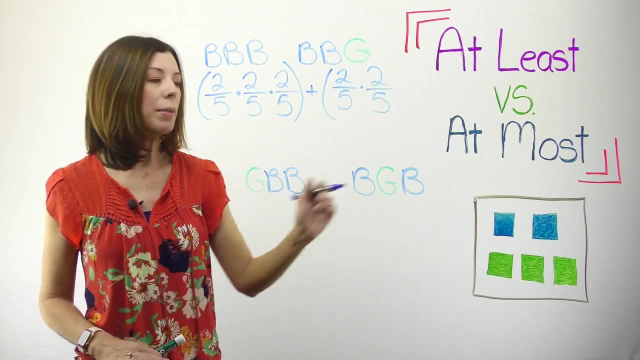 and I'm going to go to my blue, blue, green. So again I have two-fifths and I'm going to be adding these together, So two-fifths times two-fifths. And then, if I look at my green, 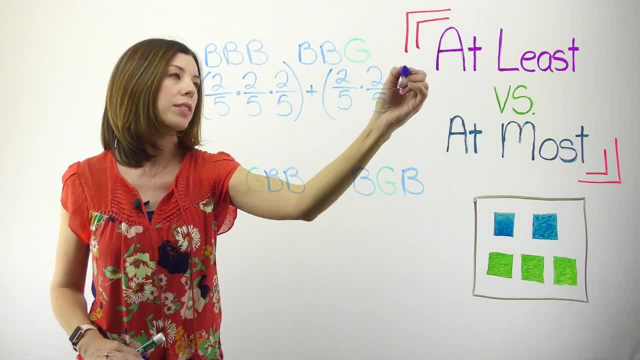 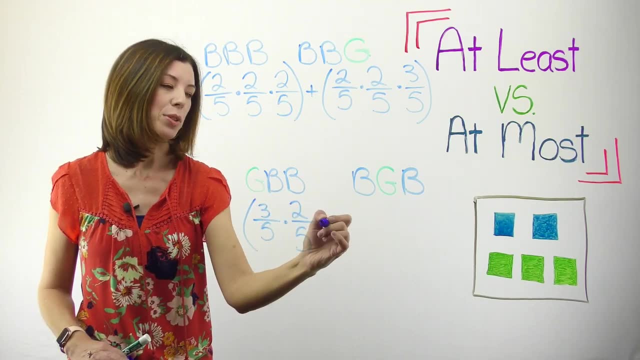 I can see that I have three out of five, So times three-fifths. Now I'm going to go down here to my green, blue, blue. I have three-fifths times two-fifths, times two-fifths. 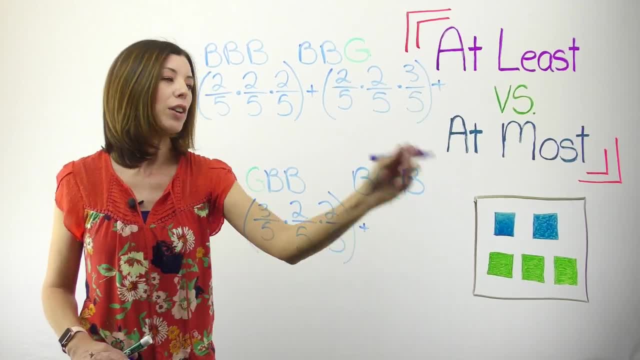 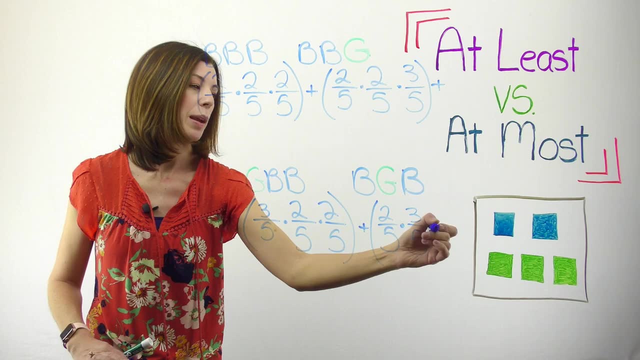 Again, I'm going to be adding these. And then, lastly, I've got my situation of a blue- two-fifths Times my green, which is three-fifths Times my blue, which is also two-fifths. 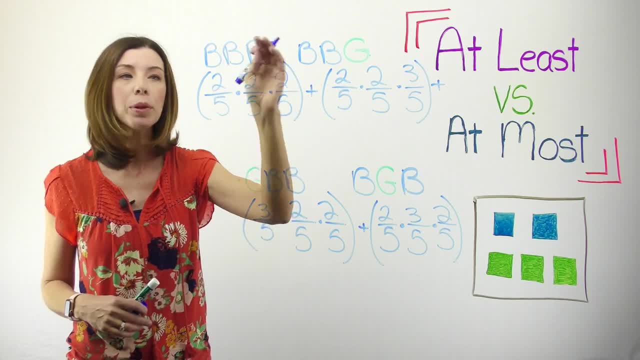 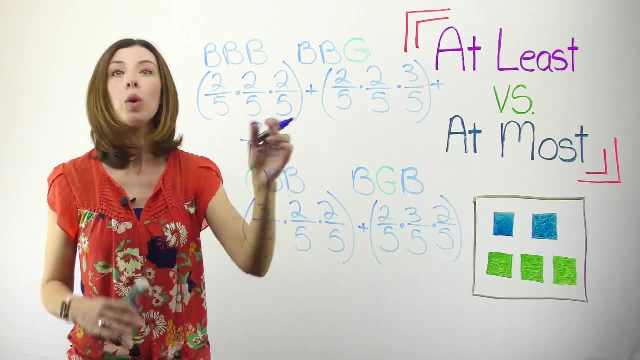 You can see that I'm going to find the probability for getting a blue blue blue, which is going to be eight, one-hundred-twenty-fifths. Okay, five times five times five would be one-hundred-twenty-five. 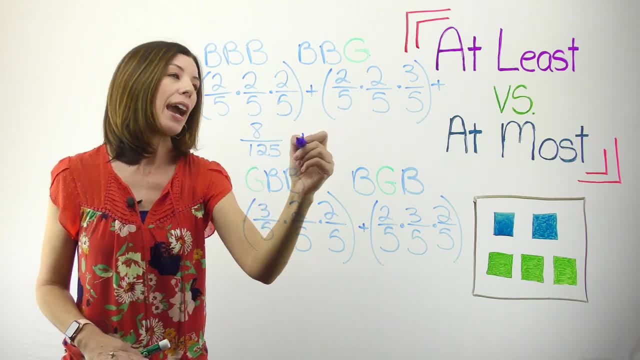 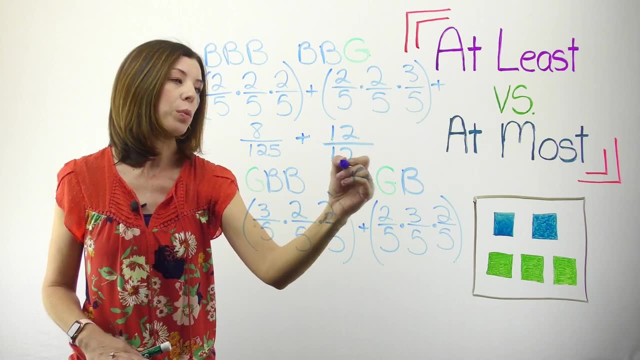 Two times two times two or two-cubed would be eight. I'm going to be adding that to two times two times three, which is going to be twelve, And again five times five times five, over one-hundred-twenty-five. 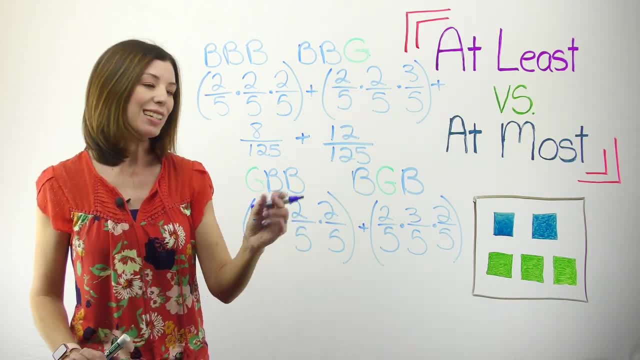 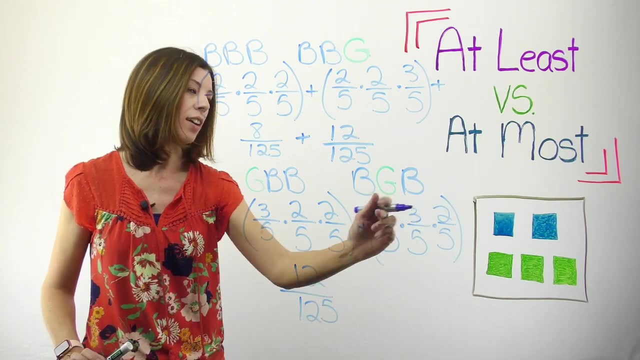 So twelve, one-hundred-twenty-fifths, And then next I'm going to do three times two times two, which is going to give me twelve, one-hundred-twenty-fifths, And then I have two times three times two. 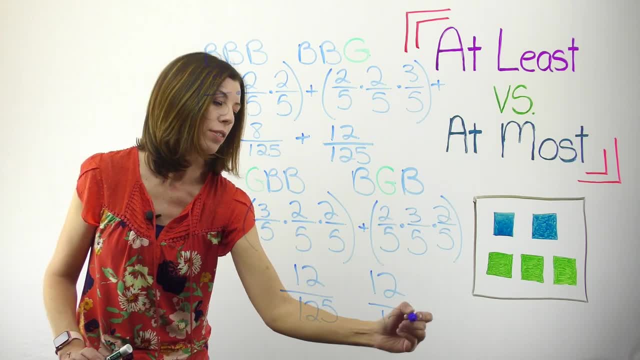 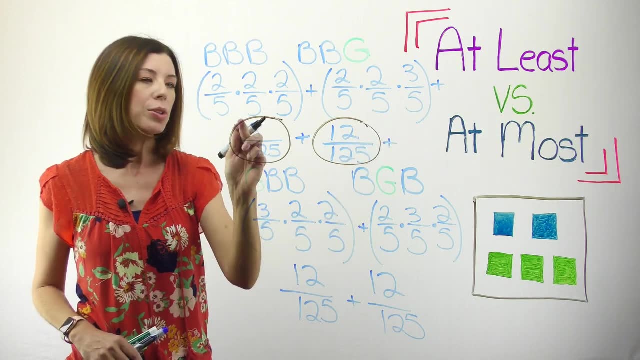 which is going to also give me twelve one-hundred-twenty-fifths. So I'm going to be adding all of these probabilities here, my situational probabilities. So I have eight one-hundred-twenty-fifths, twelve one-hundred-twenty-fifths. 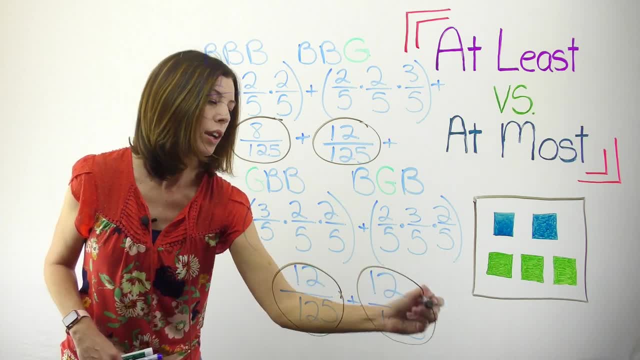 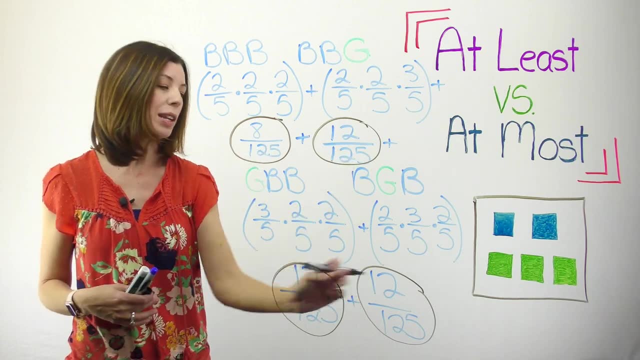 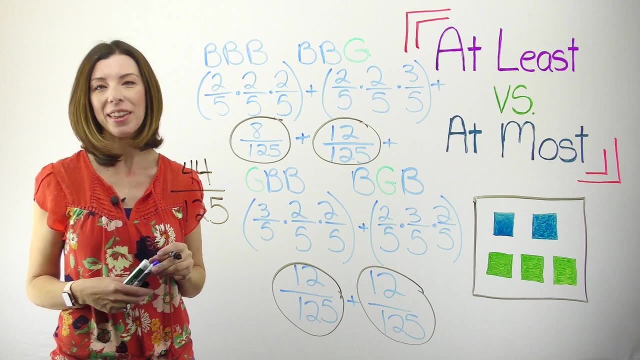 twelve one-hundred-twenty-fifths and another twelve one-hundred-twenty-fifths. When I add these all together, you can see that I have the exact same common denominator. so that's awesome. Three groups of 12 IC, which is 36, plus an additional 8, would give me 44 125ths. 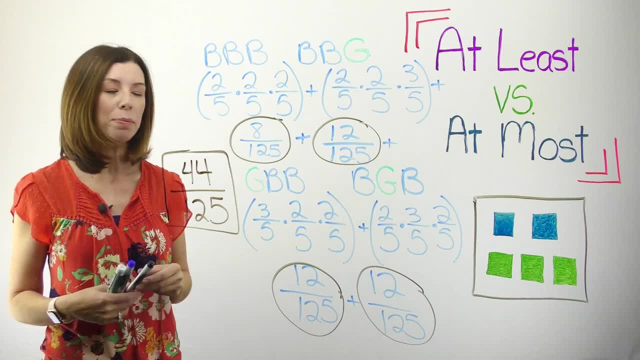 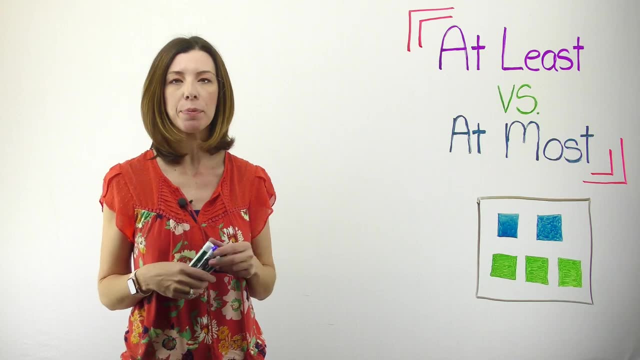 My probability for getting at least two blue cubes would be 44 125ths. Okay, so let's recap for a moment and kind of think through how we solve this problem. The first thing we needed to do is we needed to list the potential outcomes where we're.